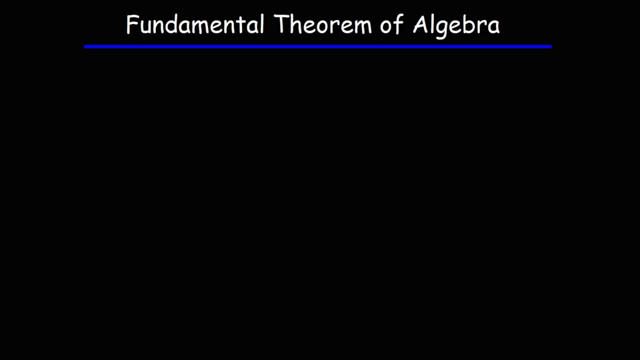 In this video we're going to talk about the Fundamental Theorem of Algebra. What is the Fundamental Theorem of Algebra and what can it help you to do? Let's say you have a polynomial p of x that has a degree n, where n is equal to or greater than 1.. 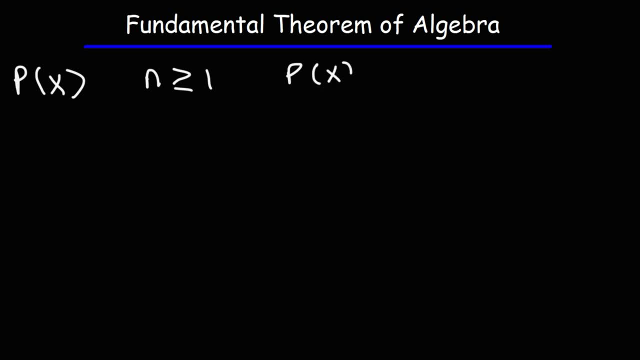 If you set that polynomial equal to 0,, then that polynomial has exactly n roots. So n can't be 0 or a negative number. As long as n is 1 or larger, then whenever that polynomial is set equal to 0, it's going to have n roots. 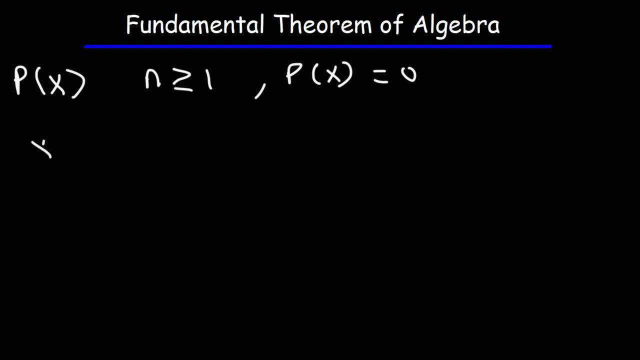 So here's an example. Let's say, if we have a linear polynomial x minus 5.. And we set that equal to 0. This is of degree 1.. There's only one solution. If you were to graph y equals x minus 5, it would look like this: 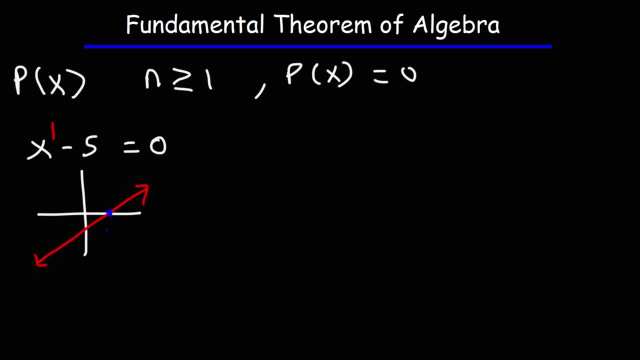 It intersects the x-axis at one point, in this case at 5.. If you solve the equation, you're going to get the root x equals 5.. So, because we have a degree 1 polynomial, there's exactly one root. In this case, we have a degree 1 polynomial. 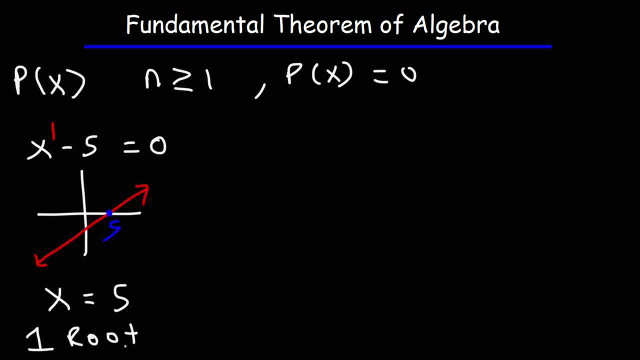 In this case we have a degree 1 polynomial. In this case, one real solution. Here's another example. Let's say, if we have the equation, y is equal to x squared minus 4.. This is a parabola that has been shifted down 4 units. 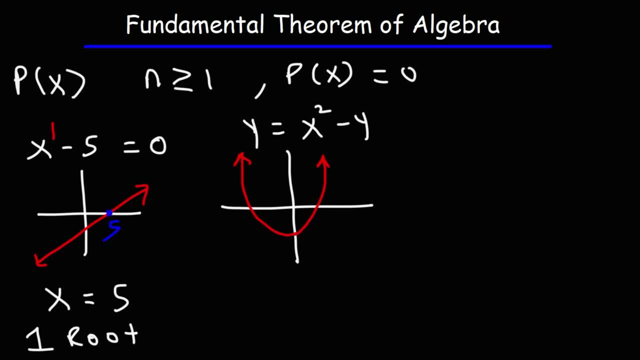 It's going to look like this. Notice the degree of this parabola: It's degree 2.. So n is equal to 2. Which means it has exactly 2 roots. So there's two solutions to this equation And we can see that based on where the graph touches the x-axis. 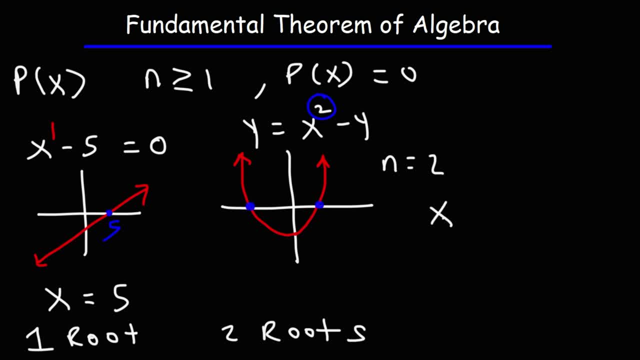 It touches it here and here. So if we set p of x, this is going to be our p of x If we set it equal to 0.. So if we set x squared minus 4 equal to 0 and solve for x. 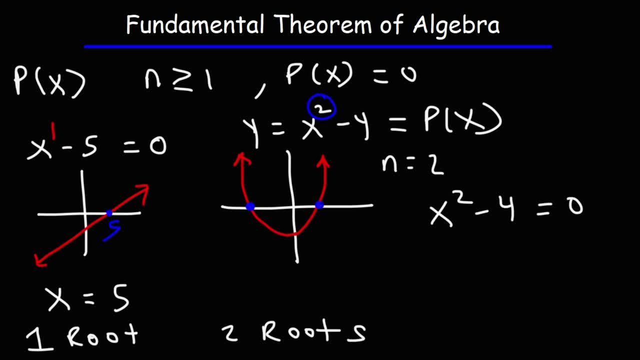 we're going to get two solutions. So we can factor it using the difference of perfect squares method. The square root of x squared is x. The square root of 4 is 2.. We get plus or minus 2.. And if you set each factor equal to 0 using the 0 product property. 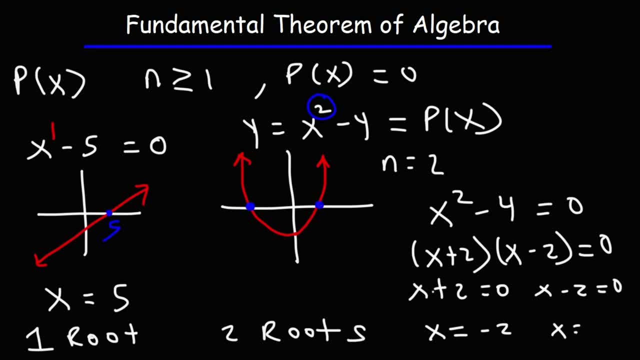 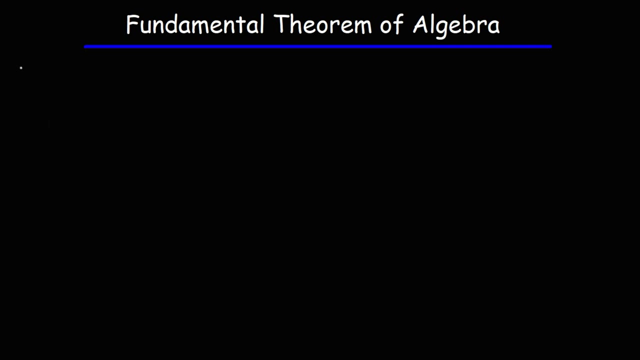 you're going to get two solutions: x is equal to negative 2 and x is equal to positive 2.. So, based on the fundamental theorem of algebra, we have a polynomial of degree 2 and we got exactly two roots. Now what about this? 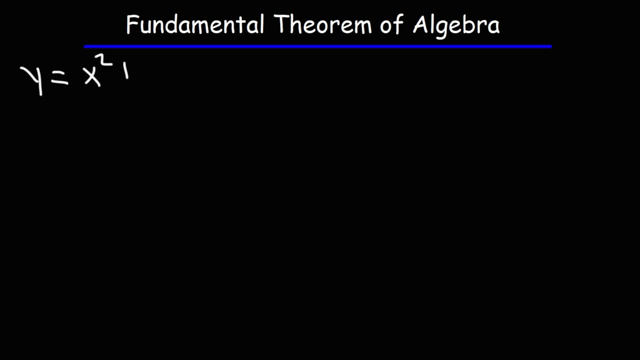 Let's say, if we have, y is equal to x squared plus 4. So we have a polynomial of degree 2. So we must also have exactly 2 roots. So we have a polynomial of degree 2. So we must also have exactly 2 roots. 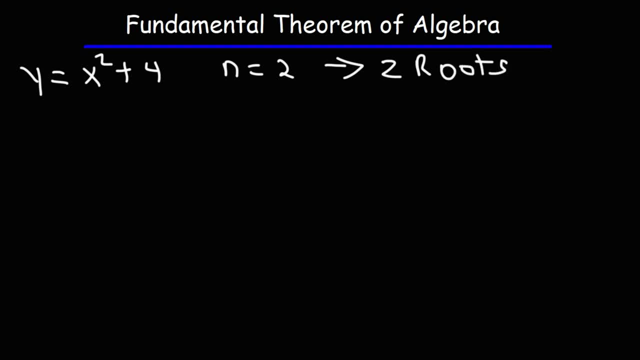 So we have a polynomial of degree 2.. So we have a polynomial of degree 2.. So we have a polynomial of degree 2.. So we have two roots in this. So we have exactly two roots or two solutions. Now, if we were to graph it, 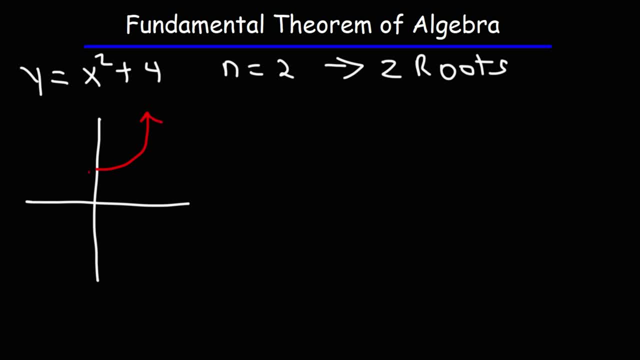 this is a parabola that's been shifted vertically up four units because of the plus 4.. So this point right here, the y-intercept, that is at 4, or 0, 4.. Now notice that this graph does not touch the x-axis. 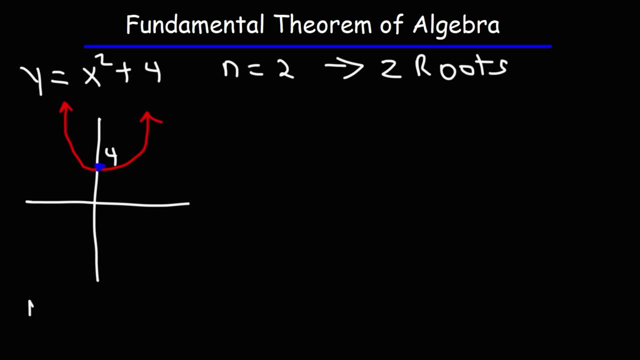 So because it doesn't intersect the x-axis. So, because it doesn't intersect the x-axis, no real solution or no real roots. but according to the fundamental theorem of algebra, we have exactly two roots and that's still true. we still have two roots, it's just those roots are not real. 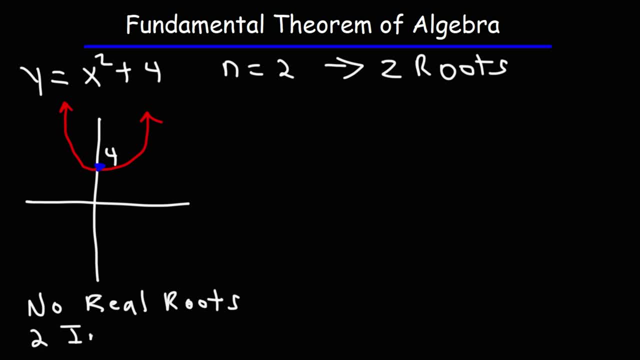 what it means is that we have two imaginary solutions or two imaginary roots. so let's set our polynomial equal to zero and let's solve for those two imaginary roots. so if we set x squared plus four equal to zero, we can't factor it like we did the last time, because we don't have a negative sign here. 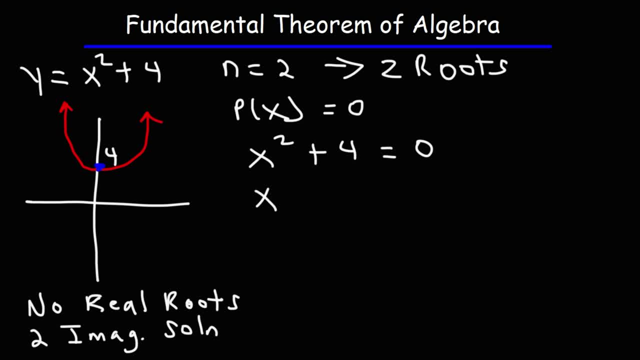 so what we need to do is move the four to the other side. subtracting both sides by four, we get x squared is equal to negative four. so next we need to take the square root of both sides. the square root of x squared is x and the square root of negative four. 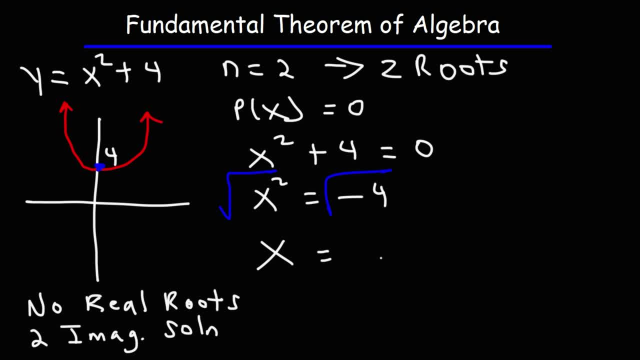 well, we're going to break it down a bit. so first I'm going to rewrite this as the square root of four times the square root of negative one, because four times negative one is negative four. now the square root of four. we can write that as plus or minus two. 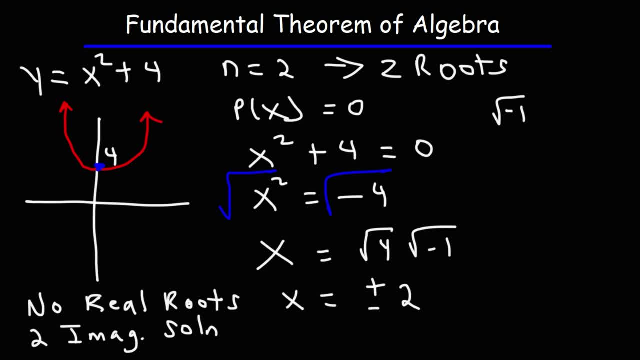 the square root of negative one. this is something you need to know. it's equal to the imaginary number i, so we get plus or minus two i, so we have two x squared minus two i. two imaginary solutions. the first one is: x is equal to positive two i. 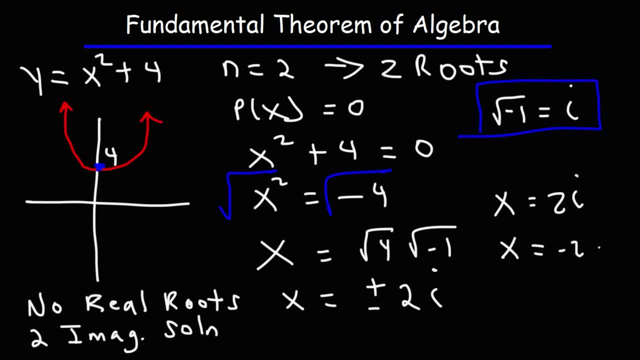 and the second one is equal to: is x is equal to negative two i. so, according to the fundamental theorem of algebra, we have a degree two, polynomial. we got two exact roots, or exactly two roots, but because the graph does not touch the, the x-axis, those roots are imaginary roots. 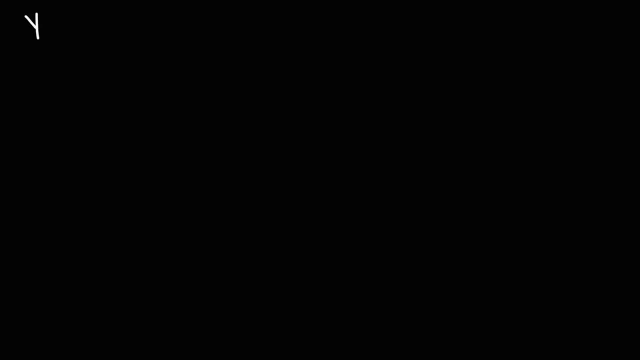 now let's say, if we have a cubic function, y is equal to x cube minus two, x squared plus X minus two. using the fundamental theorem of algebra, determine the number of roots that this polynomial has and also determine the types of groups that it has. Is it the real roots, Imaginary roots, And how much each is? 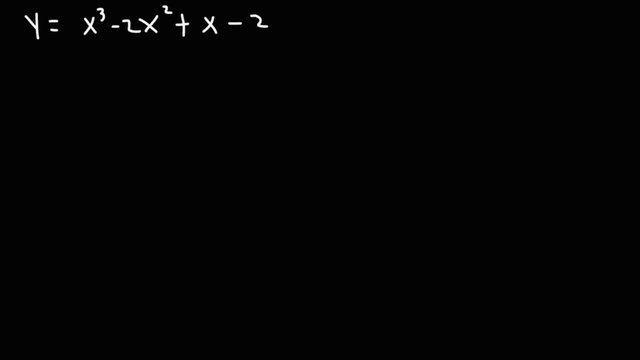 much of each of those roots do we have in this polynomial, So feel free to pause the video Now. there's two ways we could do this. We can do this analytically or graphically. Let's start analytically and then we'll confirm our answer by graph. 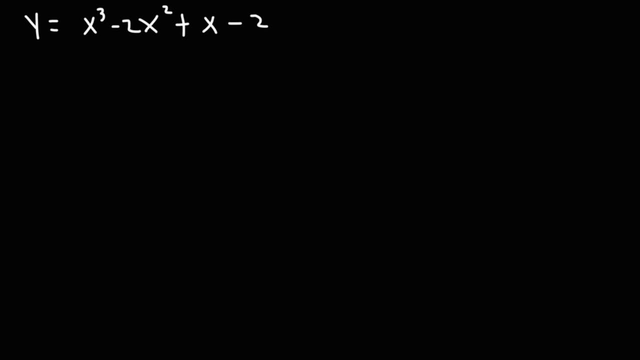 So the first thing we want to do is identify what type of polynomial we're dealing with. So we look at the highest exponent. The highest exponent in this polynomial is 3.. So we're dealing with a degree, a polynomial of degree 3,, which means this polynomial has exactly 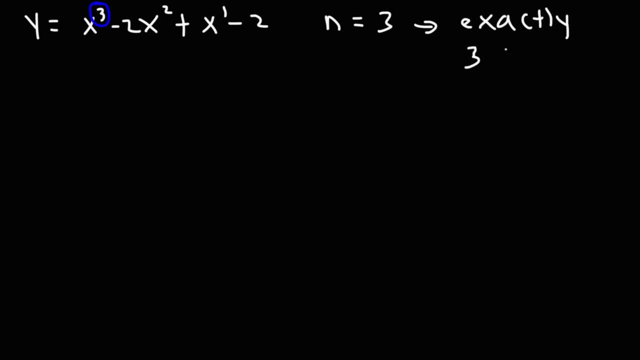 three roots, So now we need to know how many, what type of roots we're dealing with. Do we have three real roots? Do we have, or is there, any imaginary roots? By the way, imaginary roots always come in pairs, So you can't have one imaginary. 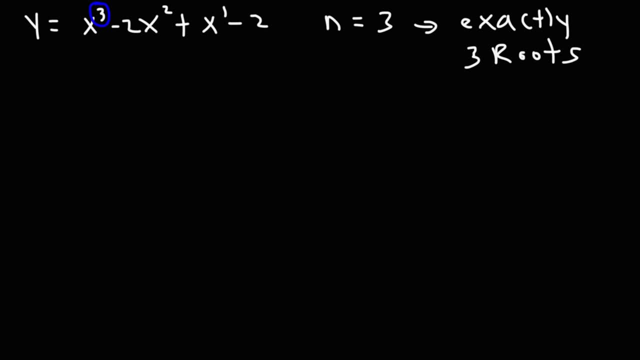 Nor can you have three imaginary roots. It's always even. You can have two imaginary roots or four imaginary roots. So let's list the options that we have With three roots. this could be three real roots and no imaginary roots. That's option one. Option two: we have one real root. 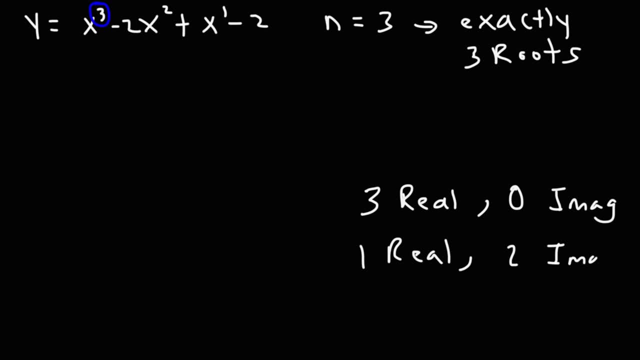 and two imaginary roots. So, with three roots, these are the only two options that we have. The question is which one? Is it option A or option B? Well, let's find out. Let's set this polynomial equal to zero. 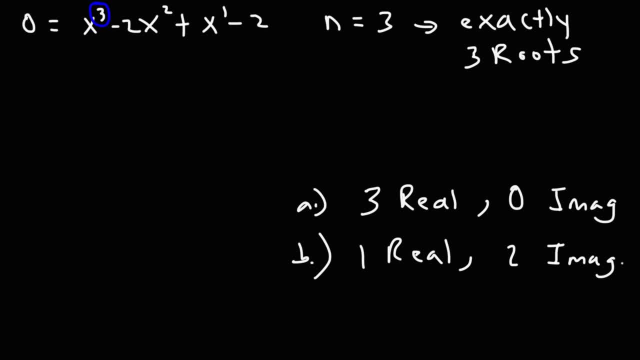 And let's factor it, Notice that the first two terms has the same ratio as the last two terms. If you look at the coefficients, this is 1, negative 2, and this is 1, negative 2.. When you see that, 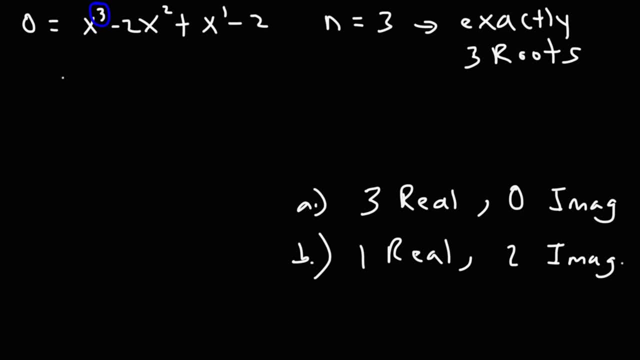 you can find out that the first two terms have the same ratio as the last two terms. So let's factor by grouping. So in the first two terms, I'm going to take out the GCF, which is x squared, x cubed. divided by x squared is x. 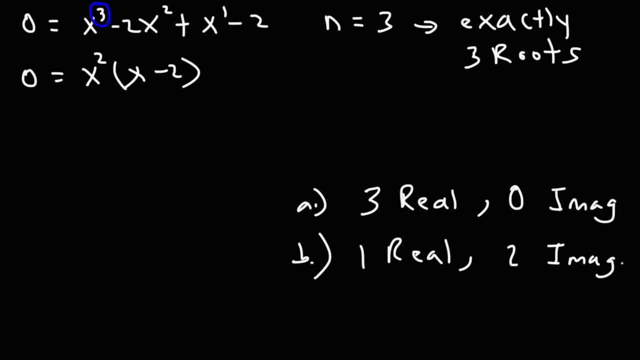 And negative. 2x squared divided by x squared is negative 2.. In the last two terms, I'm just going to take out 1.. When you take out 1, you're going to be left with x minus 2.. So now the GCF between these two terms is going to be x minus 2.. 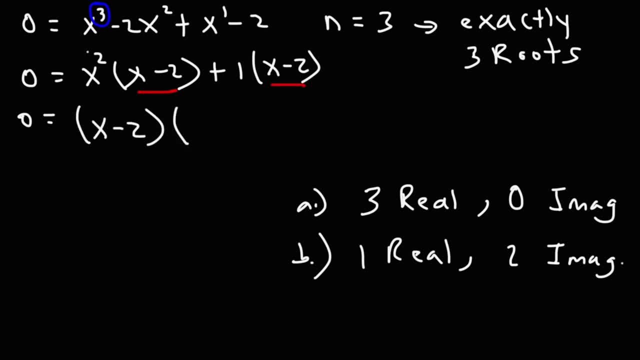 So I'm going to factor out an x minus 2, and here I'll be left with x squared. When I take out x minus 2, here I'm left with plus 1.. Now, at this point, what we can do is set each factor equal to zero. 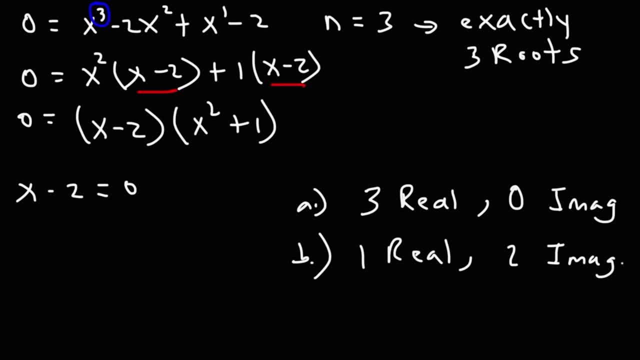 So if we set x minus 2 equal to zero, once we add 2 to both sides, we'll get our first real solution, which is x is equal to 2.. Now, if we set x minus 2 equal to 0,, we'll get our first real solution, which is x is equal to 2.. 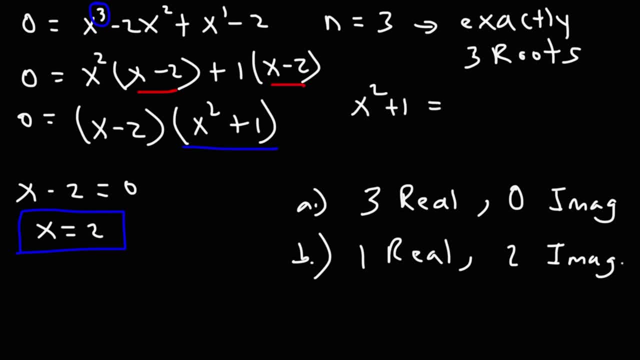 Now, if we set x squared plus 1 equal to 0, subtracting 1 from both sides, we get: x squared is equal to negative 1.. And then if we take the square root, the square root of negative 1 is going to be plus or minus i.